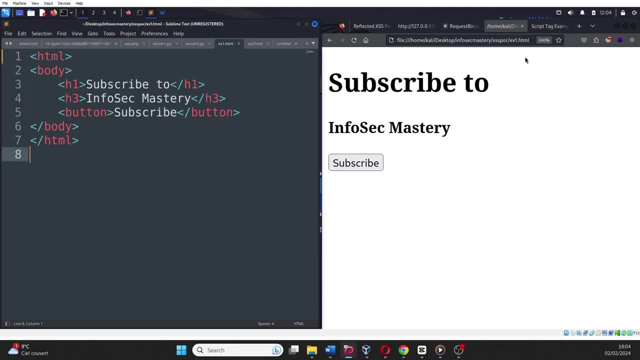 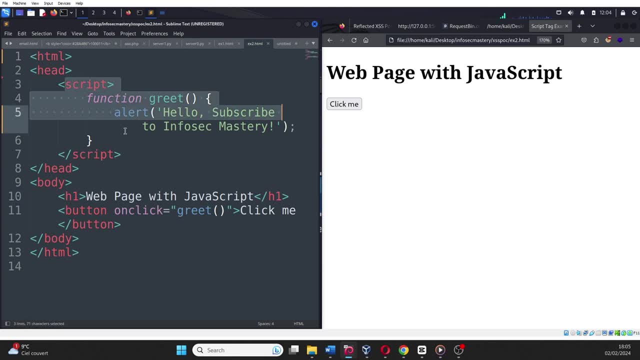 an indication for creating various content elements in HTML. Finally, let's discover the script tag in HTML. The script tag in HTML is used to embed or reference JavaScript code within an HTML document. JavaScript is a programming language that allows you to add dynamic behavior and interactivity to. 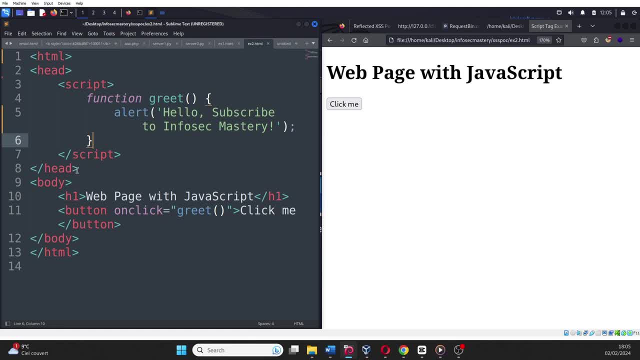 your web pages. The script tag can be placed in the head or body section of an HTML document. Here is a basic example of how the script tag is used. In this example, the script tag contains a simple JavaScript function named greet. This function displays an alert saying hello, subscribe. 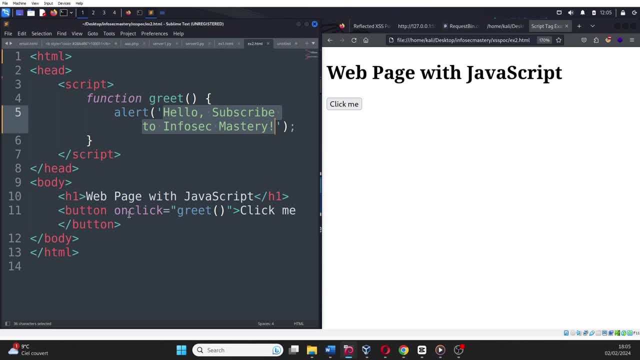 to infosec mastery. when called, The button element in the body section triggers this JavaScript function when clicked, demonstrating the interaction between HTML and JavaScript. Now, after all these shenanigans, where is the XSS attack? Just like in HTML, the script tag is used to report a new condition, ie a new object. 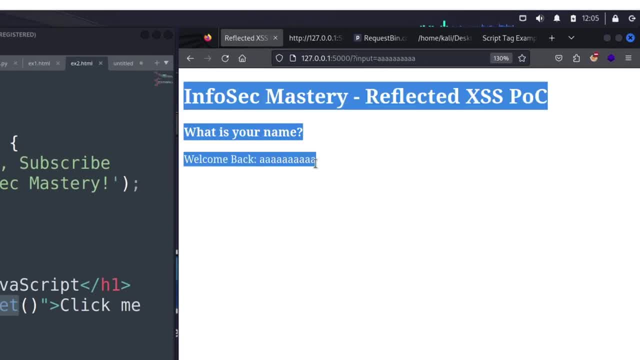 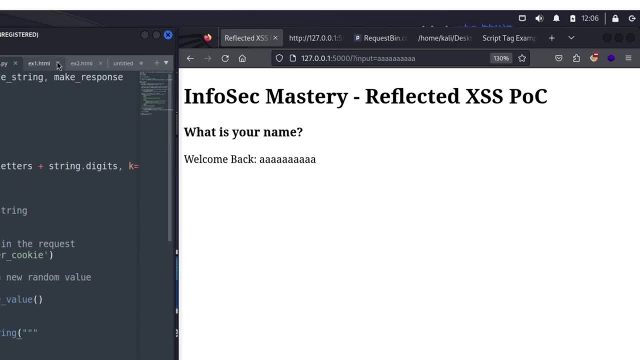 The script tag also ensures that the object is not accessed by an encore. Let's look at an example of this a bit more clearly. The script tag is a simple website that asks for your name. When you visit the main page of the website, you see a question asking. 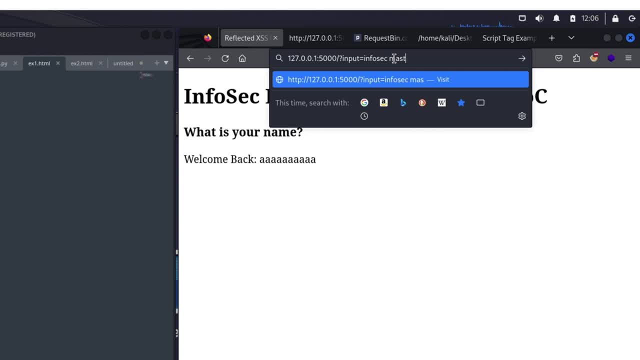 what is your name and the page is expecting you to put your name in the url for the page to display it back to you. For example, if you visit mastery on the page, The interesting thing about how webpages work is that when you add something to the page, 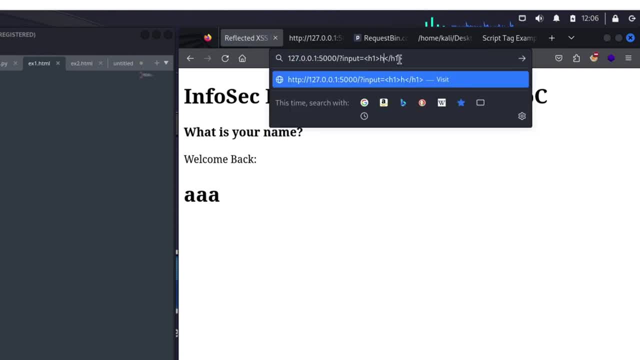 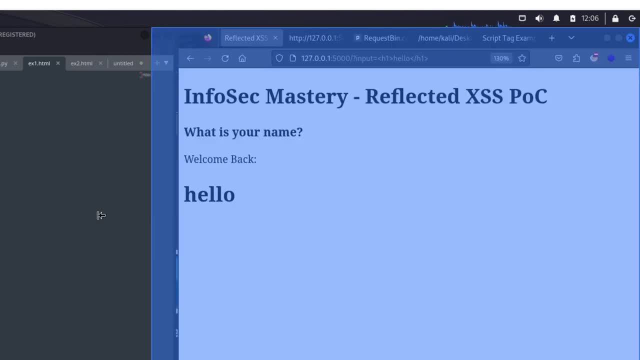 that looks like an element, it will interpret it as an element, Which means, instead of putting my name, I can put an h1 tag that says hello, And when I click enter, I can clearly see that the page didn't just simply print out. 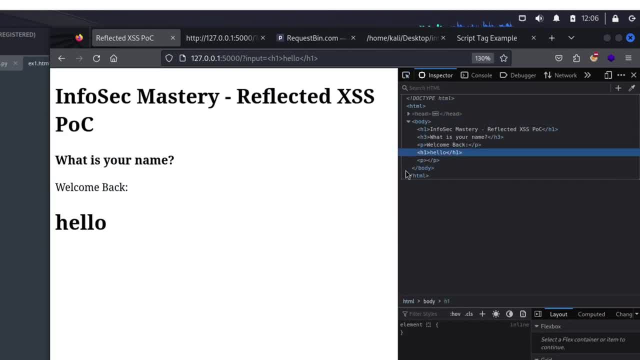 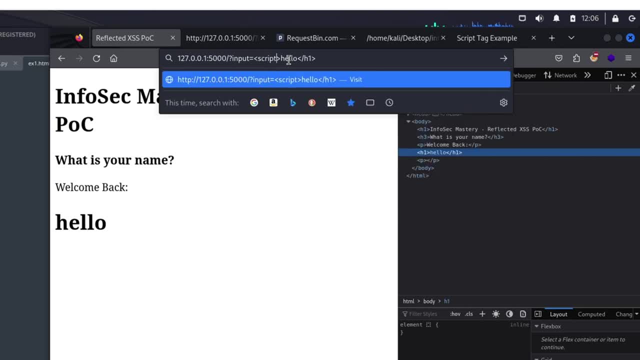 the text I gave it, but it interpreted it as an h1 tag. that's since it looks bigger to the usual text. Another interesting thing is that, instead of adding a h1 element, we can add a script element, Because, remember, script elements allow us to execute JavaScript, and executing JavaScript. 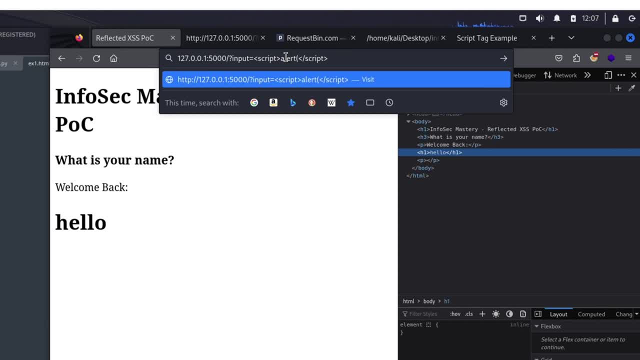 is what will allow us to perform the infamous cross-site scripting attack. To do that, it's pretty simple. We just create a new script tag, we put an alert1 function as the JavaScript code that will be executed, and then we press enter. 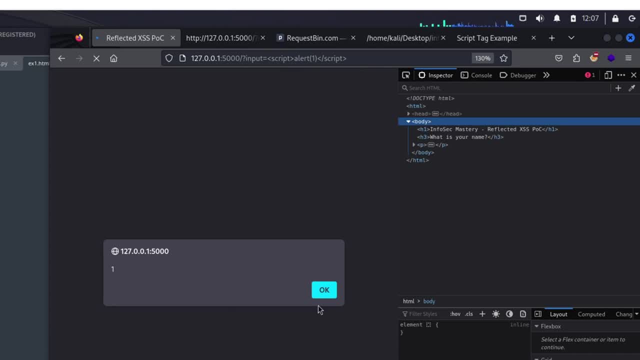 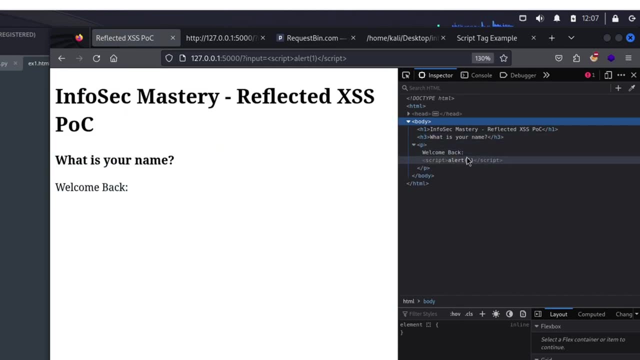 As you can see, an alert pops up in our screen with the number 1.. This in itself is a confirmation of the existence of the XSS vulnerability. Well, you might be saying it's not interesting, is it? What can we even do with this? 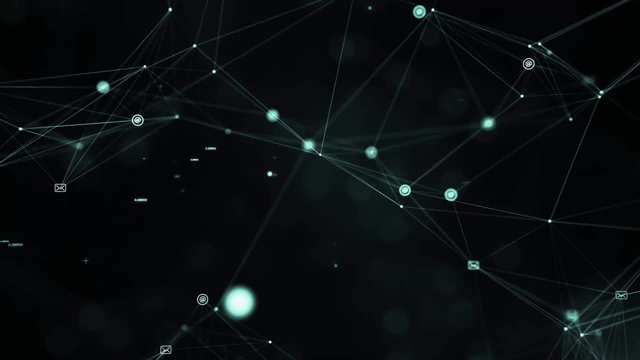 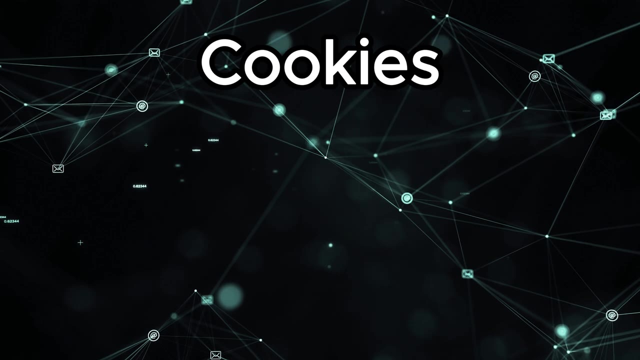 I am about to show you. just be patient with me for a second. On the website we have some things called cookies. Cookies are small pieces of data stored by websites on a user's computer. These data files serve several purposes, such as remembering user preferences, storing session. 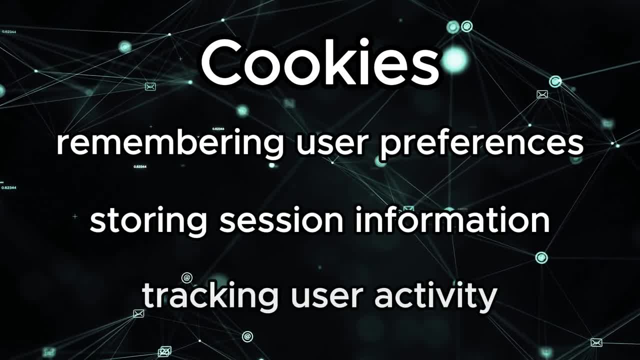 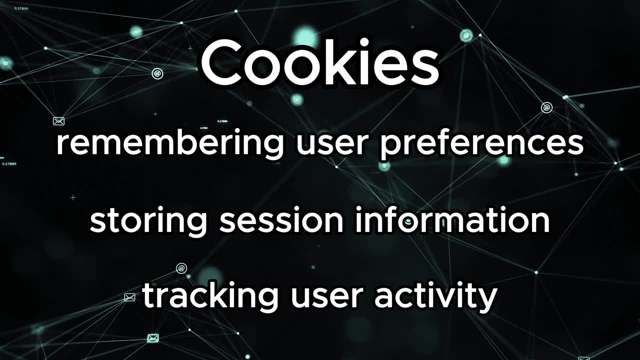 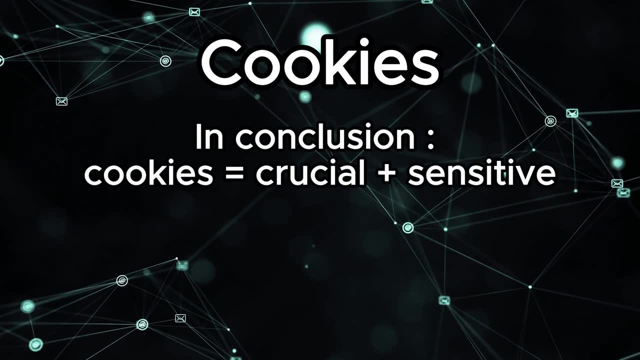 information and other things. Cookies are commonly used for tasks like keeping users logged in, remembering items in a shopping cart and customizing website settings based on individual preferences. Cookies are crucial for maintaining stateful interactions between a user's browser and a website, contributing to a smoother and more personalized browsing experience. 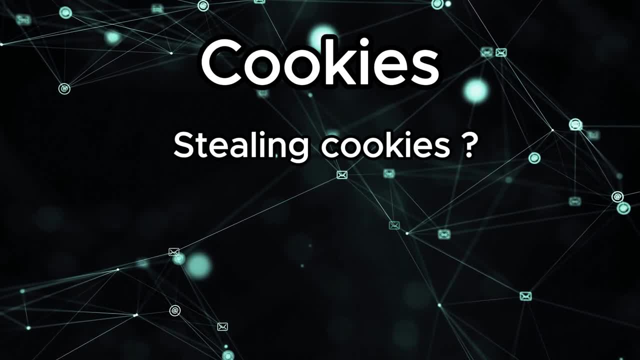 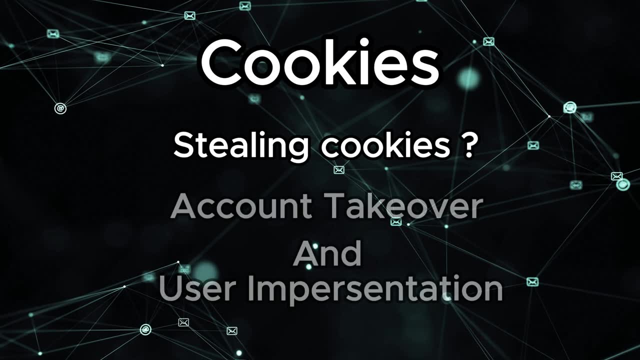 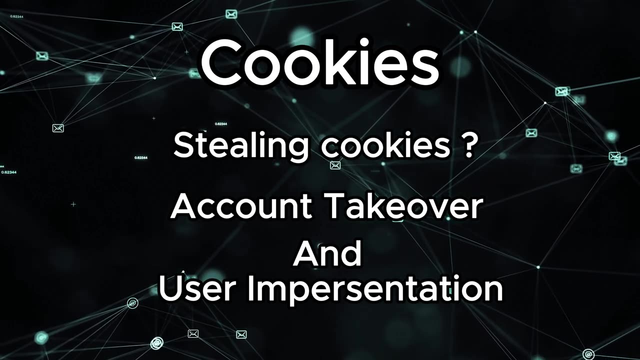 So if we can steal these cookies from other users using JavaScript, that attack would be very interesting, wouldn't it? Because when we can steal cookies, we can simply take over the account of that user just by telling the website: hey, I am the admin user and I can prove it. 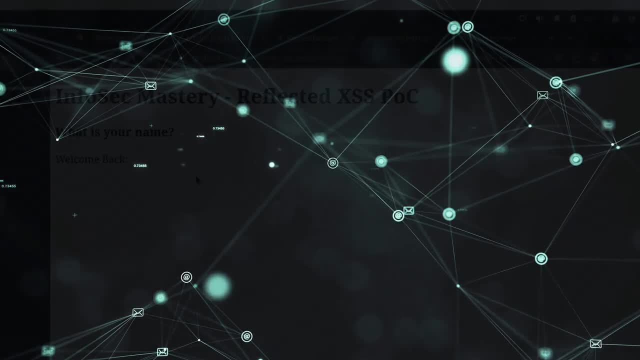 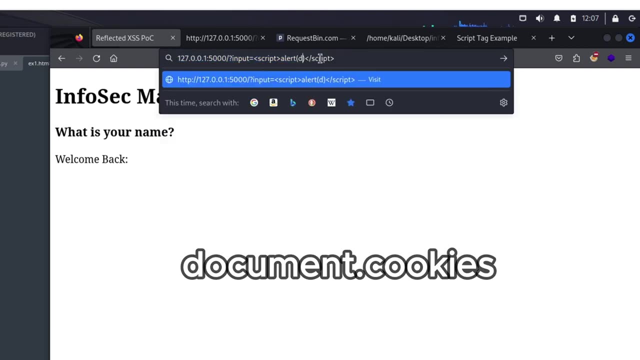 And your proof is the cookie that you stole from the admin user, of course. So the way we can do that is we go back to our XSS attack payload and we just simply swap the number 1 with documentcookie. This will print out the cookies stored for the current document, meaning the current. 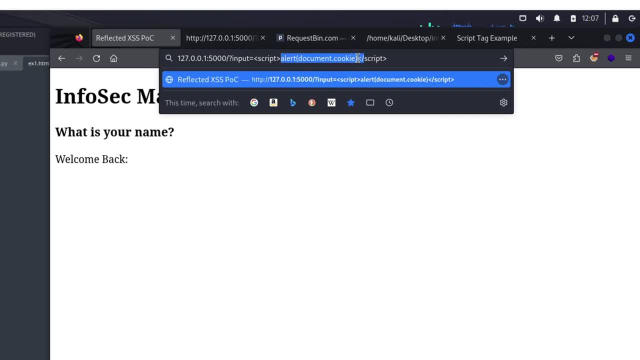 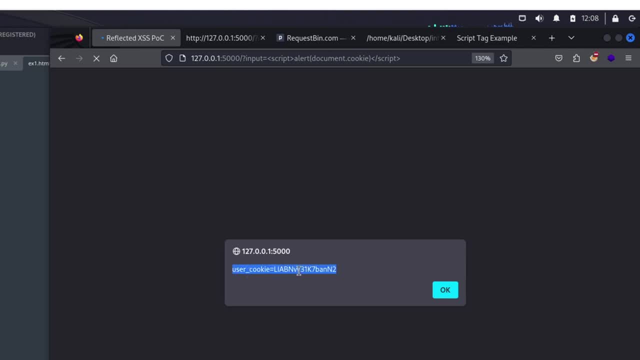 website, Hence the namedocumentcookie. When we do that, you can see that we get our usual popup, but this time it says userCookieEqual and the value of the actual cookie. So this confirms that we will be able to get the cookie through JavaScript. 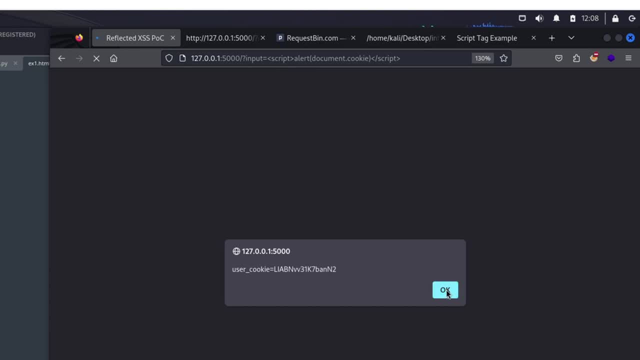 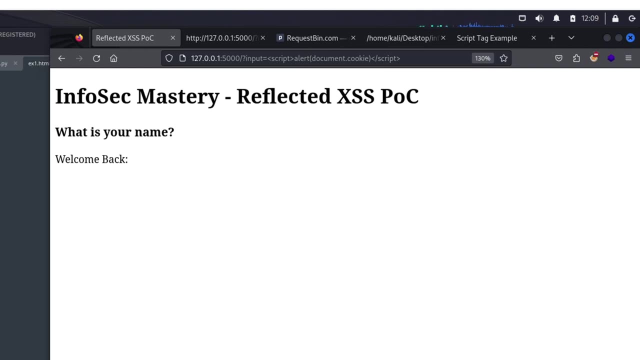 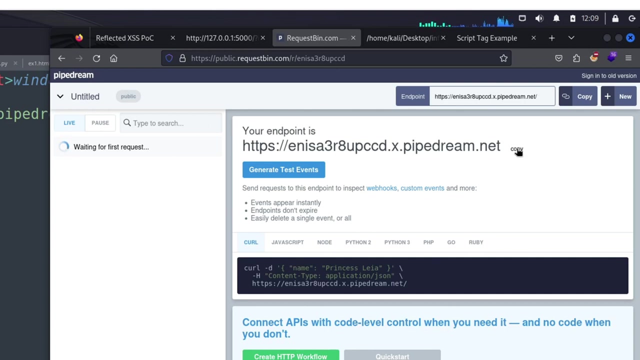 Now, how can we actually steal this cookie from a user? The simplest way is to send it to another website waiting on the other side. Let me demonstrate that Here we have a website called Requestbin. Requestbin is used to receive HTTP requests. 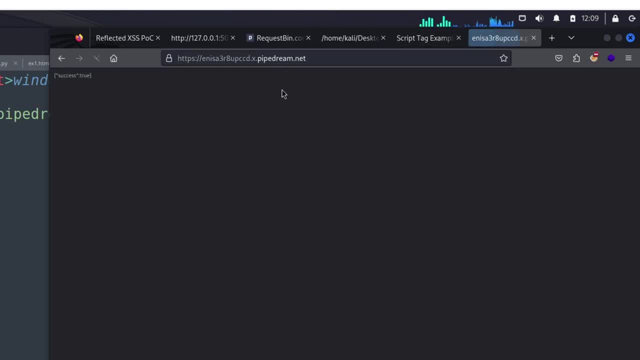 The usage is simple. You create a public bin, you get the link and then you just ping it. When you ping it, you can see that a new request is generated in Requestbin. Now we add a new parameter in the request. 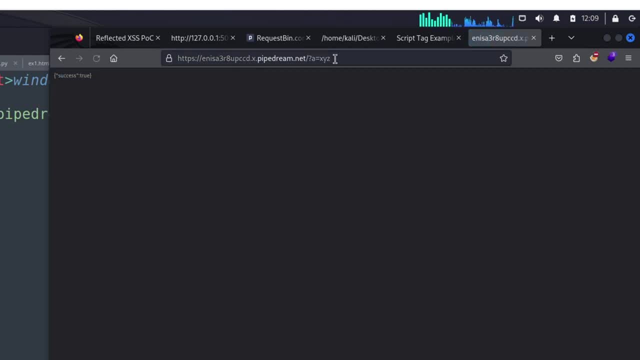 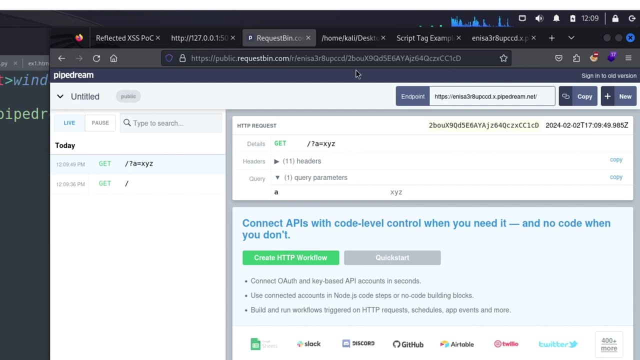 We can add a variable, a equal to xyz, and send it On the Requestbin website. we see our new request and our parameters. Now what if we go back to our vulnerable website and execute some JavaScript code? Let's see what we can do. 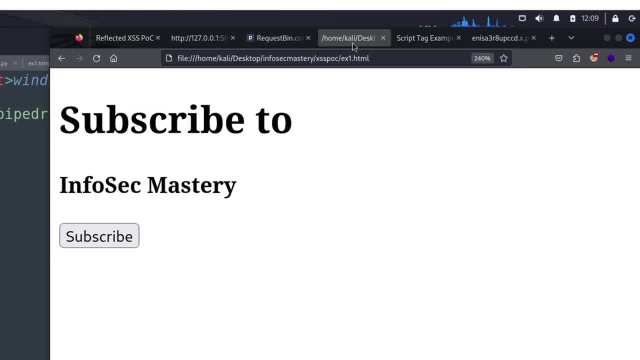 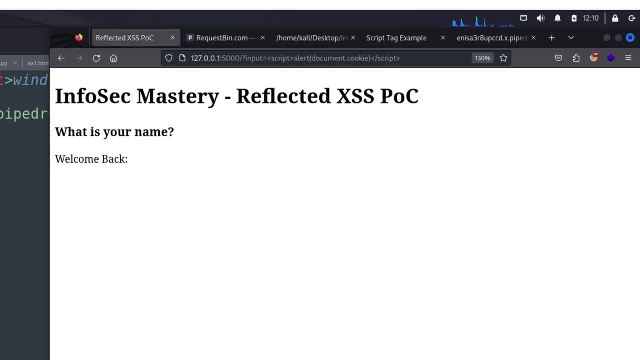 Let's see what we can do. Well, that's exactly what we are going to do In our JavaScript payload. we are going to use a redirection property instead of the alert function, which is windowlocationhref. Basically, when the vulnerable web page loads, our JavaScript code will execute and the 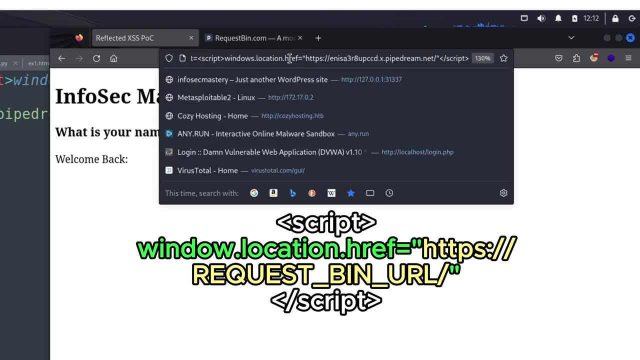 redirection property will take us to the Requestbin. We try it. we take our new payload, execute it and see that we get redirected to our Requestbin. Now, instead of just sending the cookie to our Requestbin, we are going to send the cookie. 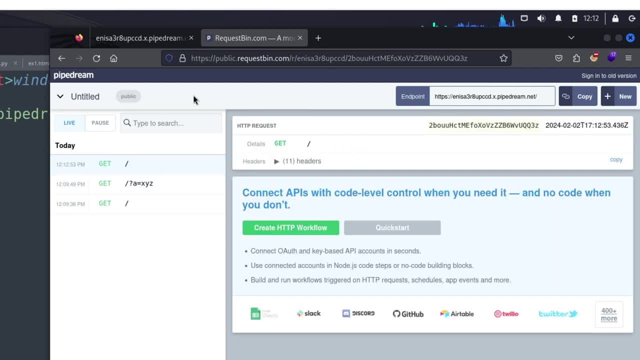 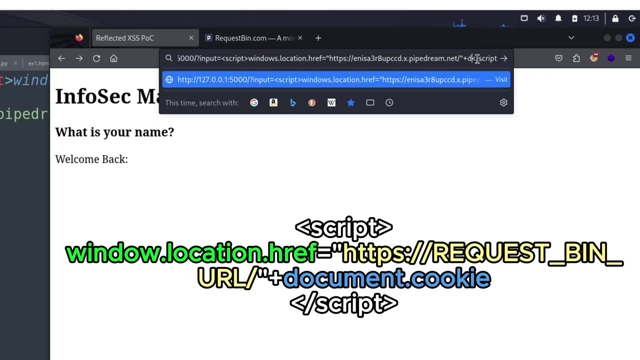 to the Requestbin. Now, instead of just making a request to the Requestbin, we are going to add the documentcookie that was explained earlier, So we just concatenate documentcookie to our redirection URL. In URL encoding, the plus character is encoded as a %2b symbol. 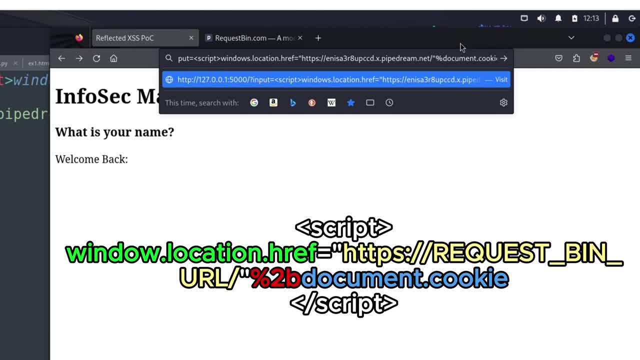 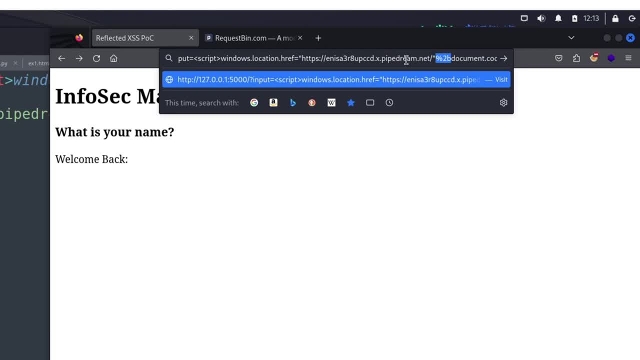 This encoding is used to represent special characters in a URL, ensuring that they are transmitted correctly and don't interfere with the URL structure. So if you have a plus character that needs to be included in a URL structure, you can use the %2b symbol. 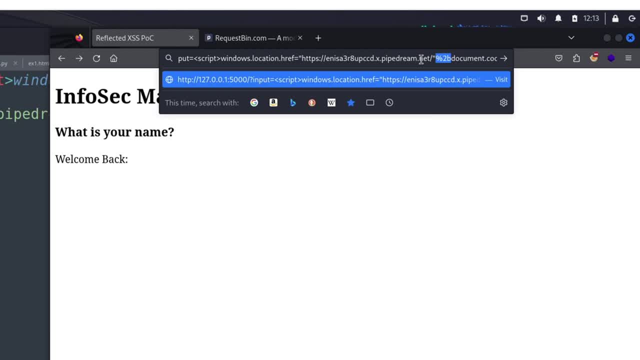 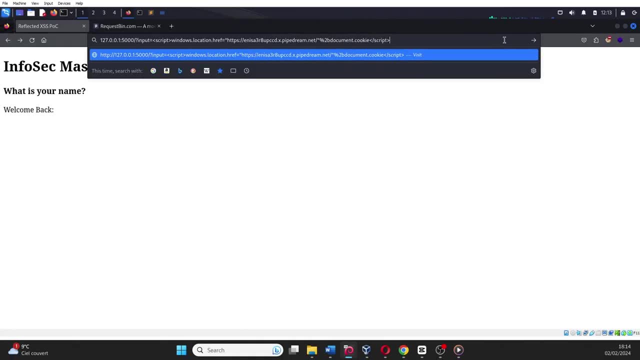 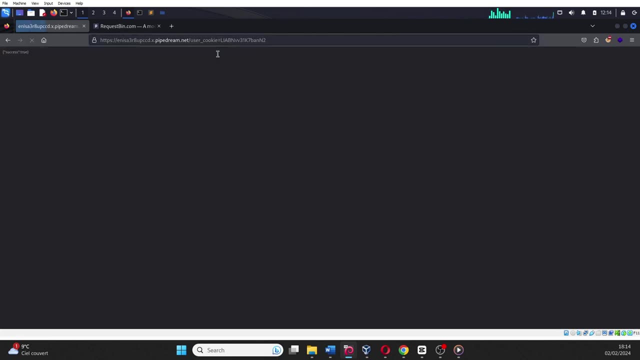 If you don't know what I am talking about, I made a video on encoding if you want to check it out. Anyways, we now take our newly created XSS cookie stealing payload, run it and see the results. On our application, we can see that we have been redirected. 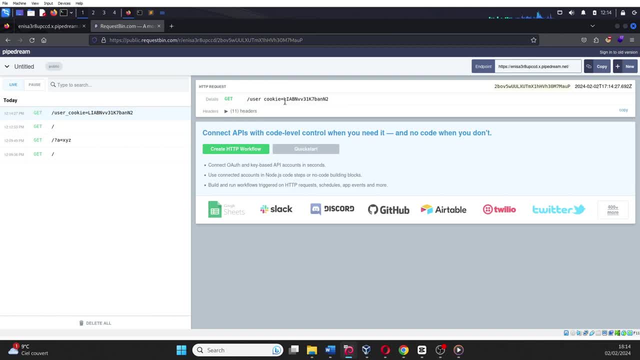 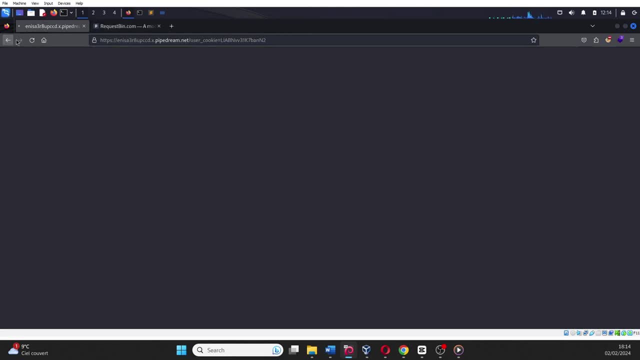 And when we check the Requestbin we see that the session cookies have been sent as well. In this case we have sent our own session cookies to request bin, which doesn't really make sense because they are our own cookies, So an attacker can give this specific link to any victim.